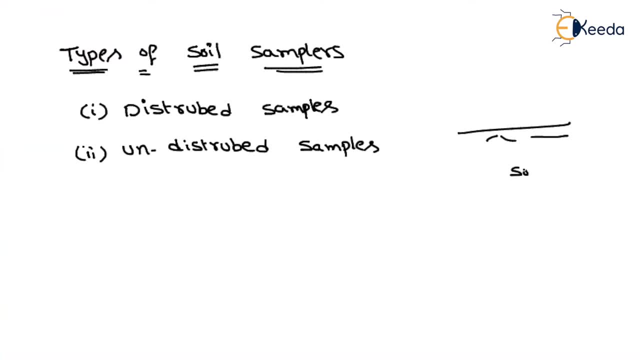 a some soil structure, isn't it? that means dispersal structure or flocculated structure. every soil is having their own structure and also every soil is having their own mineral content and also every soil is having on their water content. with respect to these three parameters, we are going to decide. 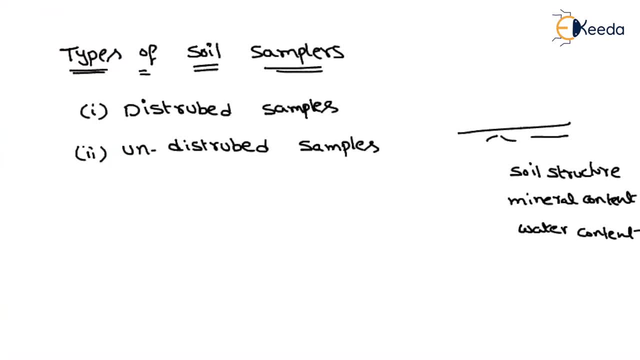 whether it comes under disturbed samples or it comes under undisturbed samples. so first let us talk about the undisturbed samples, after that we go for the disturbed sample. okay, suppose, if i am talking about undisturbed samples, undisturbed samples that means the name itself. undisturbed, that means 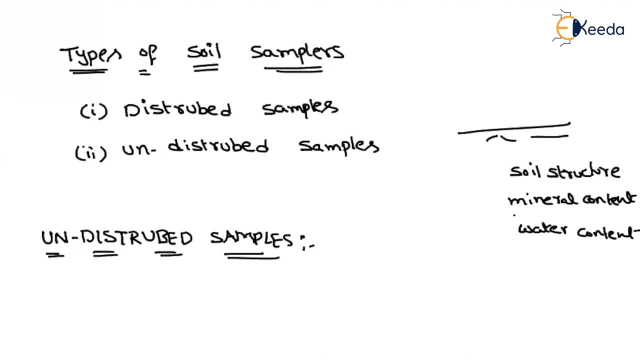 the soil structure will not change, the mineral content will not change and the water content also will not change. that means we can say: if soil structure, soil structure, mineral content and also water content, in technical term we will call it as a moisture content- moisture content are unaltered. 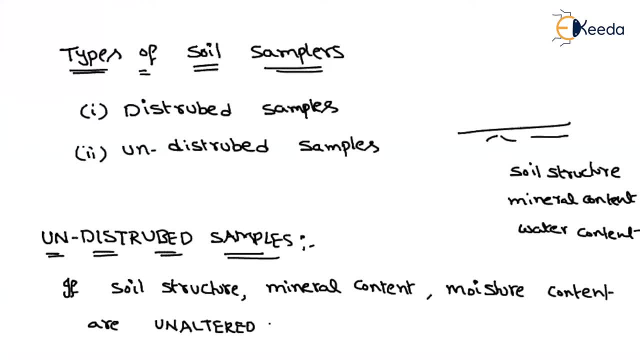 unaltered. that means this soil structure, mineral content and moisture content are remains the same. remains same when after the collection, after the collection of soil. so what we'll do? we'll use some like open method borings. by using those methods, we will dig out the soil. 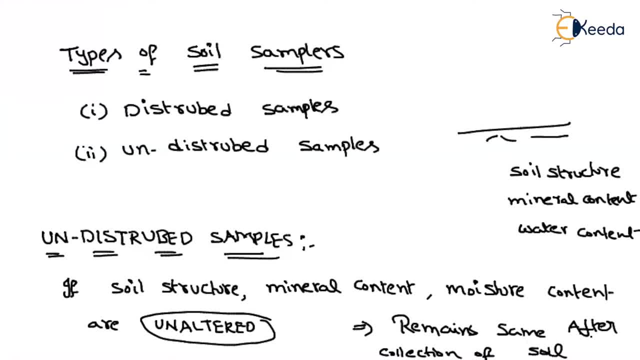 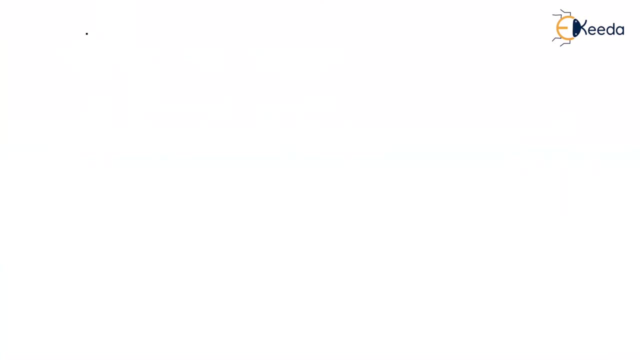 if the soil is having the same soil structure, mineral content and moisture content, we will call that as a undisturbed sample. do you really think in reality everything will be remains same? no, there will be some alteration. in reality, that means there will be some small disturbance will be there, even though the small disturbance is there in reality. whatever the method you use, whatever the sampler you use, you don't get the exactbetween mineral contents. all the واgamoth that iséstitles information semble se av handleri Mic banyak và ang gros vedäți corriété là la mentekvana, vous everlasting outgaat. intermediate moisture content are unè. c'est bardise. in reality, whatever the method you use, whatever that sampler you use, you don't. 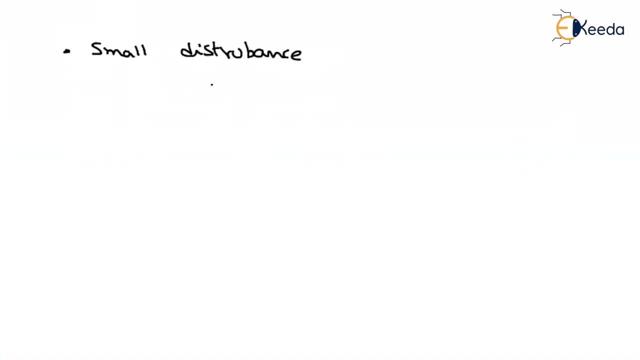 get the exact undisturbed samples. definitely there will be some disturbance, even though there will be some distance. we will ignore that. how much the disturbance? until that is not required for gate exam. only have to remember that soil structure, mineral content and water content, they will not remains change. they will remain same, even though there will be. 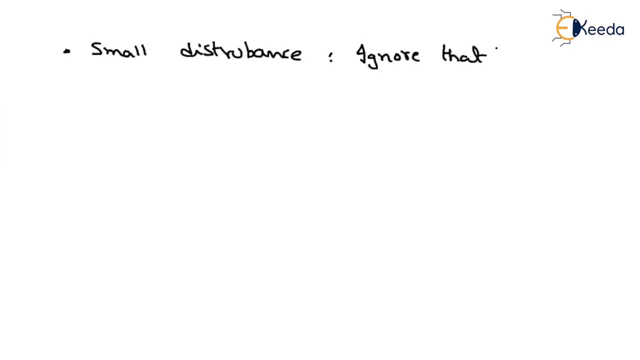 a small disturbance that we won't count into calculation part. so those type of soils we will call it as a undisturbed samples. now let us talk about the disturbance samples. disturbance samples- so here this disturbance samples also- can be divided into two categories. those are the representative samples. 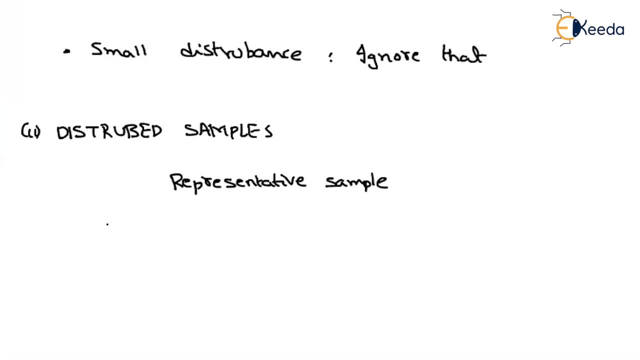 representative samples and the undisturbed samples. now let us talk about the undisturbed samples, samples and non-representative samples. non-representative samples. so in representative samples, soil structure is modified, but mineral content and water content remains unchanged. that means it the soil structure will be changed. 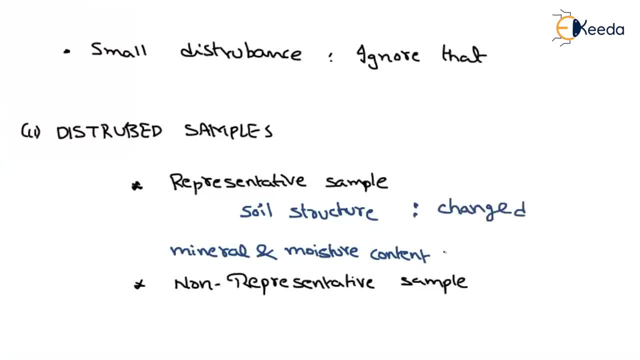 But verśa. So if your mineral and moisture content are remained same, then we will say it as a representative samples. But what about non-representative samples? Similarly, we can say: soil structure, mineral and moisture content changes after collection of sample.